try to apply this multiple linear regression models. in this particular case. This is almost applicable. Now the example is not. we try to apply this variable homogeneous, equivalent to x1 and x12. But we will use aari problem and we will. you realize that when you have the same motivation. 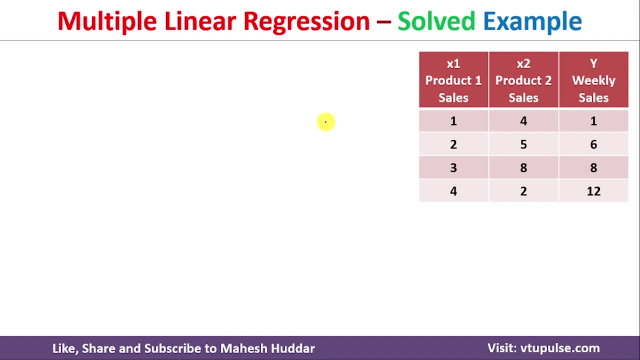 in this particular case. what you can do in this particular case is to change the valueant brush of combination dining skeptical value. We will say that we can apply the original variable, that was opinions linear regression model, on this particular data set. first we will try to write down the 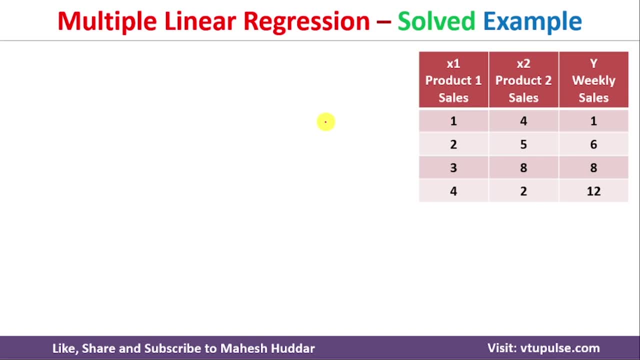 matrices for the independent variables as well as the dependent variables. the matrix for independent variable, that is x, is consisting of one column, for the bias, that is the first column, is always bias, which consisting of one. over here, the second column is nothing but the first independent variable, that is x1. over here in this case you can see 1, 2, 3, 4. we have. 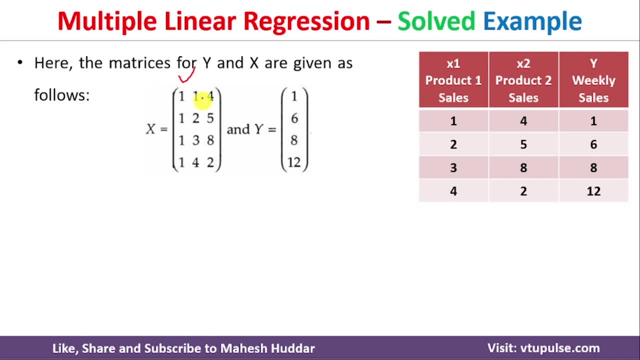 here the same thing i have written in this particular case. the next column is for the next independent variable, that is x2. it contains 4, 5, 8, 2- that is what i have written over here- and y is the dependent variable. in this case we have 1, 6, 8, 12 over here. it may be linear or 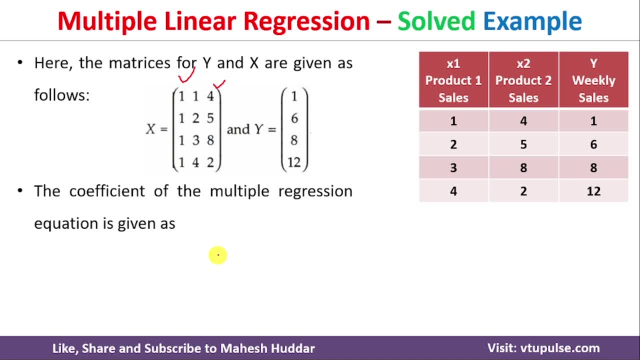 multiple linear regression model. in both the cases we need to calculate the coefficient of the bias, that is, x1 over here and x2 over here, and x2 over here and x2 over here. coefficients: the first one is something called as a intercept, that is nothing but a0. a1 is a. 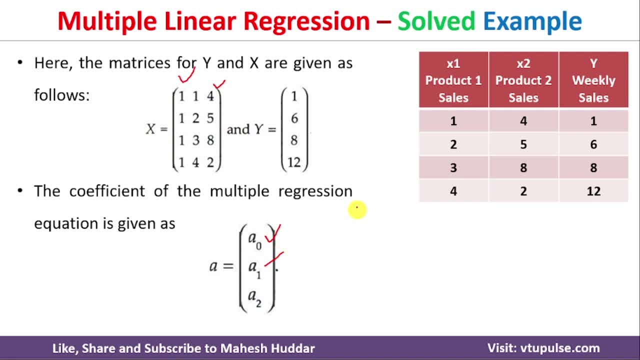 coefficient of first independent variable. in linear regression model we have only one independent variable, so we need to calculate only a0 and a1. but when it comes to multiple linear regression model, we need to calculate the coefficients based on the number of independent variables. in this case we have two independent variables, so we need to calculate. 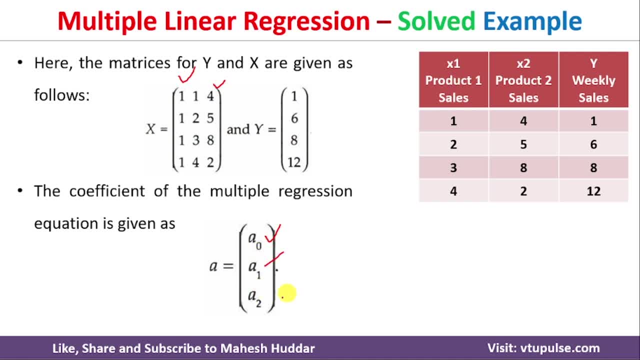 a0, that is intercept. a1 is a coefficient of x1. a2 is a coefficient of x2 in this particular case. now the question comes in front of us: how to calculate these values, that is, a0, a1 and a2. again, it may be a linear regression model or multiple linear regression model. 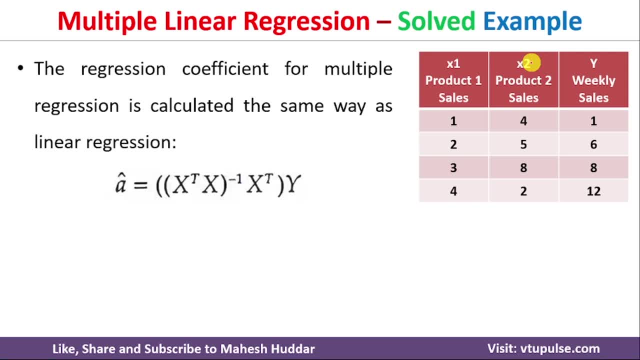 we use this particular equation, that is matrix, a is always equivalent to x transpose multiplied by x inverse. so first we need to calculate this particular term and then we need to multiply this particular intersection inverse term with x transpose, and then we need to multiply this with y over here. once you do all. 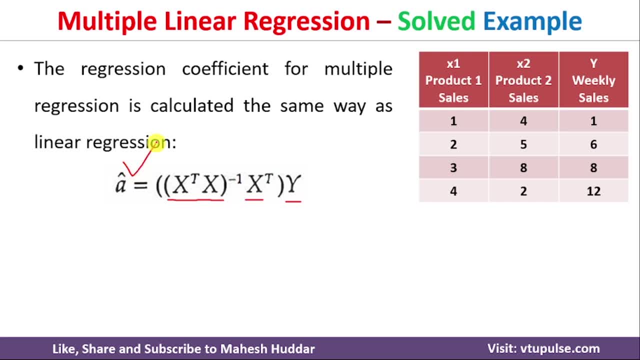 these party things. you will get that particular a matrix over here that is a, 0, a, 1, a, 2 and so on. now we will try to solve this particular equation step by step. first we will try to get the value of x transpose multiplied by x. here we know what is the value of x. we will convert that particular. 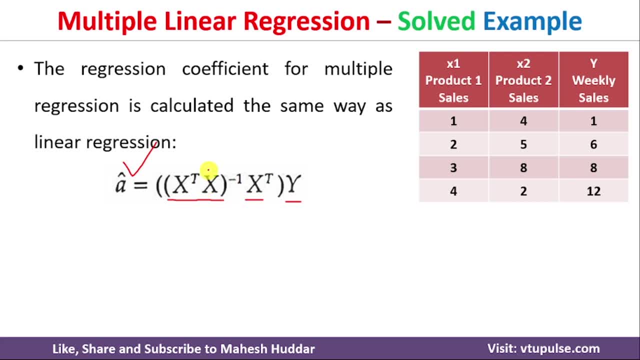 x into x transpose. that is, each of the column will be converted into rows over here. so this is what x over here: the columns are converted into rows. in this particular case, we have three columns, so we got three rows in this particular case. now what we need to do is we need to multiply. 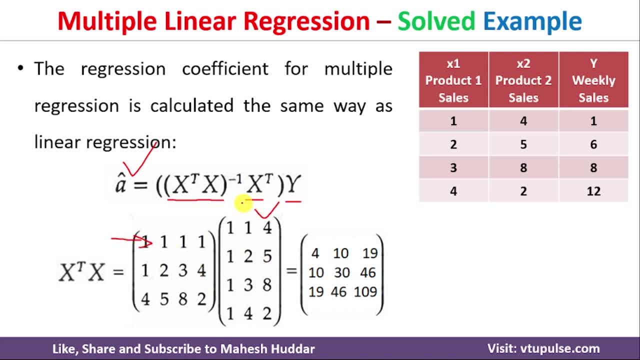 these two matrices, the this row is multiplied to this particular column to get this particular four over here. that is 1 into 1 plus 1 into 1 plus 1 into 1 plus 1 into 1. that is nothing but four over here. similarly, the same row is multiplied to the second column: 1 into 1 plus 1 into 2 plus. 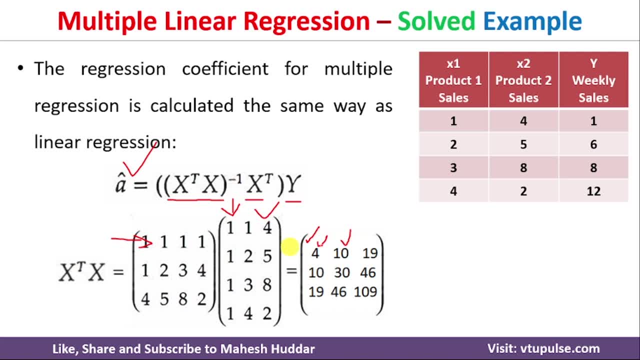 1 into 3 plus 1 into 4, that is nothing but 10 here. similarly, we need to calculate all other possibilities over here. so once you calculate this particular thing, we will get this x transpose multiplied by x over here. this is the matrix, what we have calculated in the previous step. step now we need to calculate. 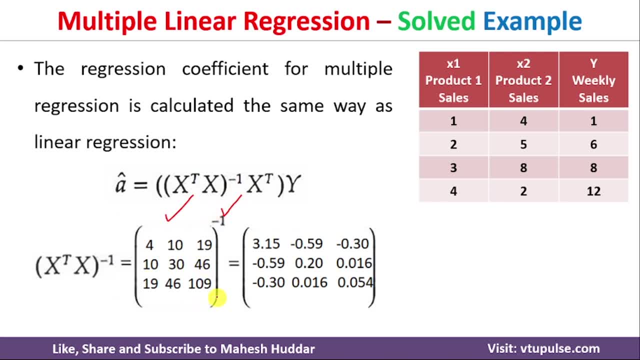 inverse, so you can easily calculate this particular inverse using your scientific calculator. put this particular values and then get the inverse of this particular calculation, so you will get the inverse. something like this: that is, x transpose, x inverse is equivalent to this one. the meaning is we got this particular entire term. 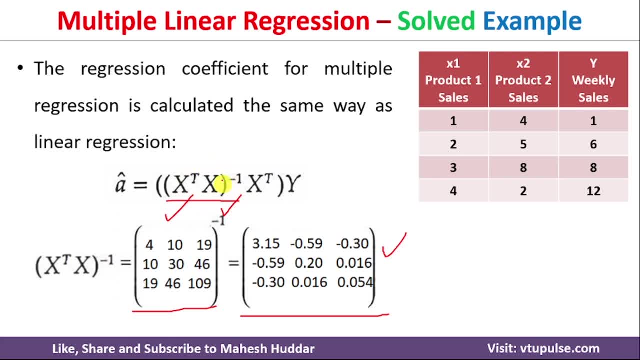 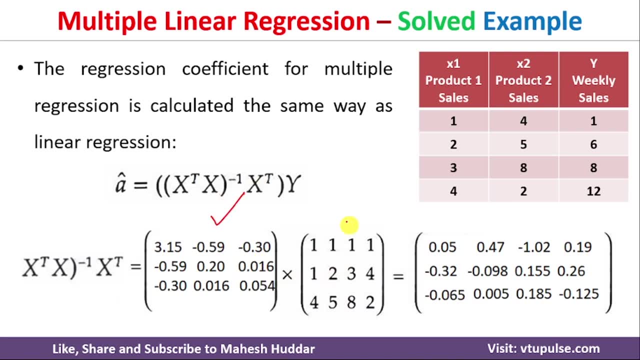 here now what we need to do. we need to multiply this particular term to this particular x transpose. so we have already calculated this one. now this one will be multiplied to x transpose. once you multiply this to x transpose, we will get this particular matrix. so this is a 3 by 4 matrix. 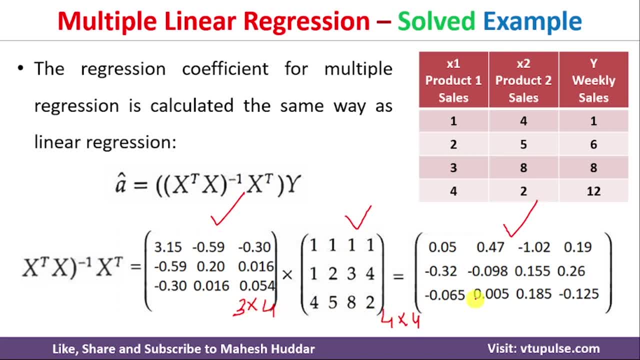 this is a 4 by 4 matrix, so the final result will be by 4 matrix over here. so again the same thing. you need to multiply rows to the columns and you will get this particular matrix over here. once you get this particular matrix, that is, x transpose x. 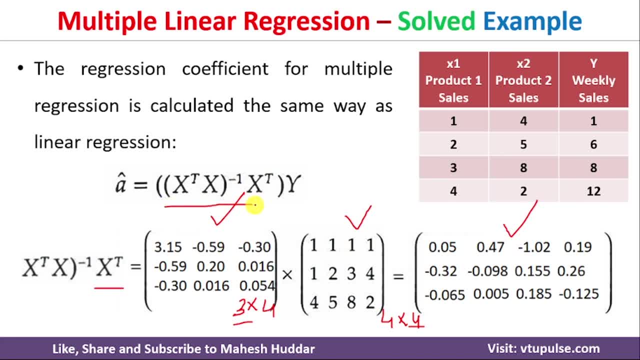 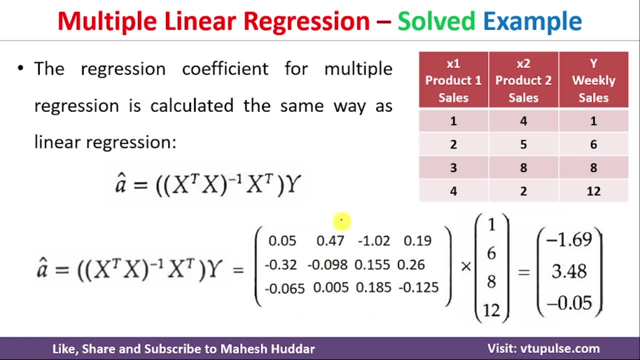 inverse multiplied by x, transpose: we need to multiply this entire matrix to this particular y that is the dependent variable in this case. so that is done in this particular slide. this is what we have calculated in the previous slide. this particular matrix will be multiplied to the dependent variable matrix. this is 3 by 4 matrix and this is 4 by 1 matrix. so the result will be: 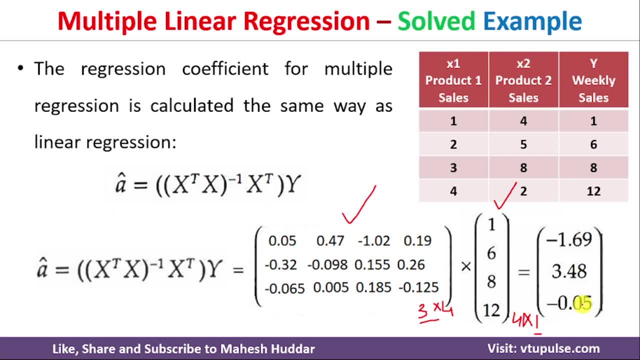 3 by 1 over here. that is, 3 rows and 1 column in this particular case. so once you multiply this particular row by column, we will get this one. this row is multiplied to this column: we will get this one. the third row is multiplied to this column: we will get this particular value over here. 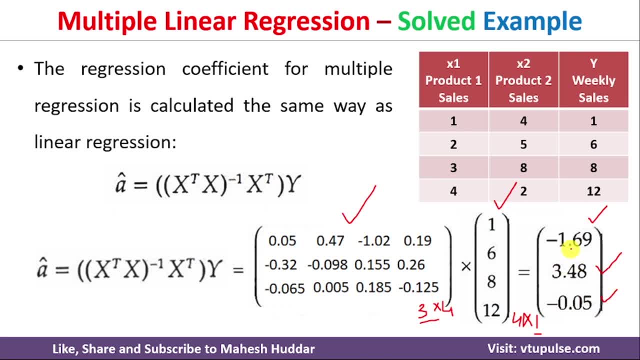 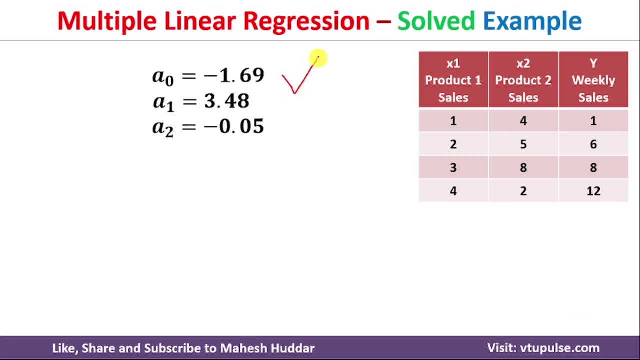 this is a 0, this is a 1 and this is a 2. so that is what i have written in this particular slide over here. now what we need to do is we need to put this particular values, that is, a 0, a 1 and. 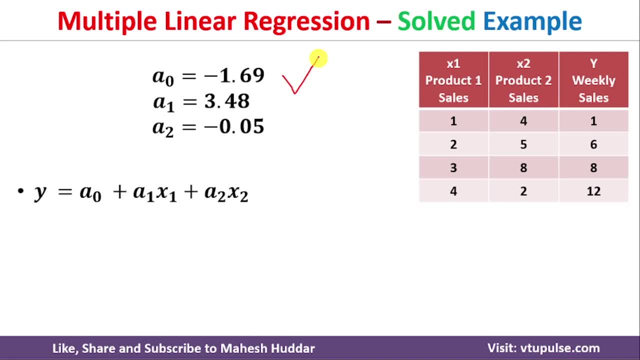 a 2 into multiple linear regression equation. this is the multiple linear regression equation. over here, y is equivalent to a 0 plus a 1 x 1 plus a 2 x 2. once you put this particular values into this particular equation, the final multiple linear regression for the given data set. 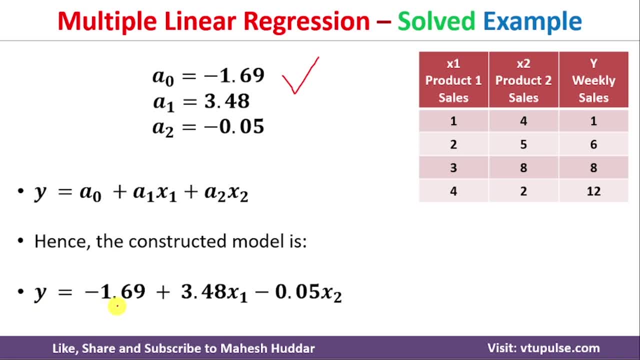 looks something like this: y is equal to minus 1.69 plus 3.4 into x 1 minus 0.05 x 2 in this case. so once you get this particular final regression equation, if you know the independent variables, that is x 1 and x 2, you can easily predict the value of dependent variable, that is y in this. 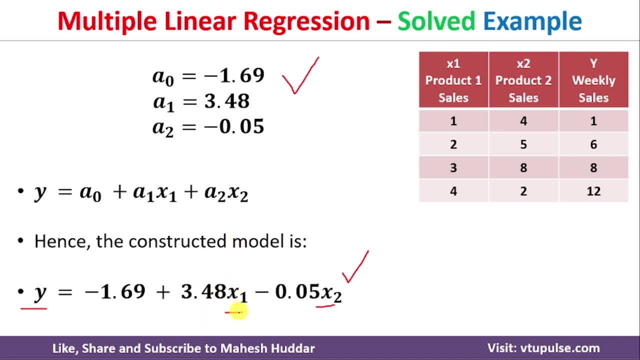 particular case. so if you know the value of x is equal to 10 and y is equal to 10, you need to put it over here. you will be able to predict the value of y with this particular model in this case. so in this video i have discussed how multiple linear regression model is different from. 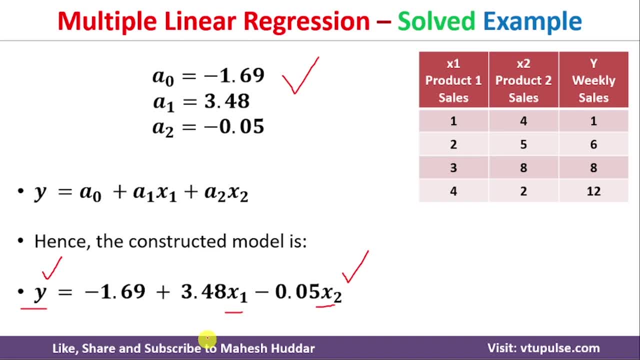 linear regression model with a simple numerical example. i hope the concept is clear. if you like the video, do like and share with your friends. press the subscribe button for more videos. press the bell icon for regular updates. thank you for watching.